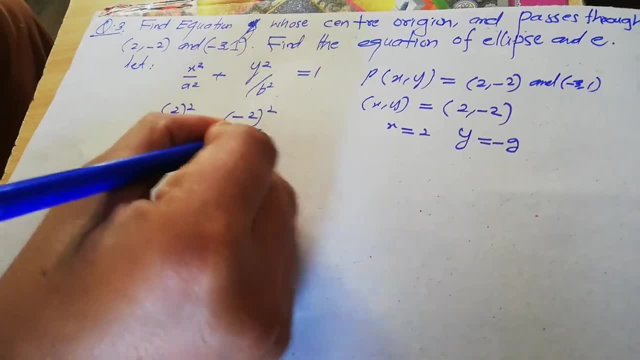 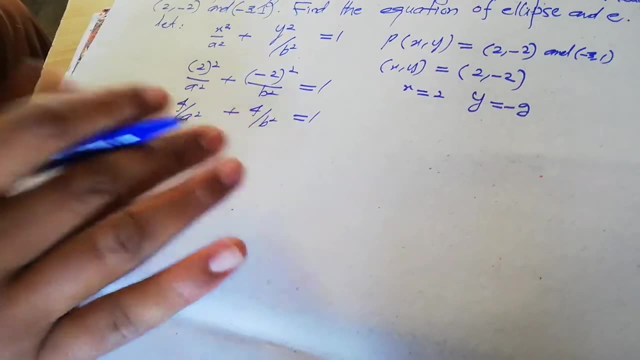 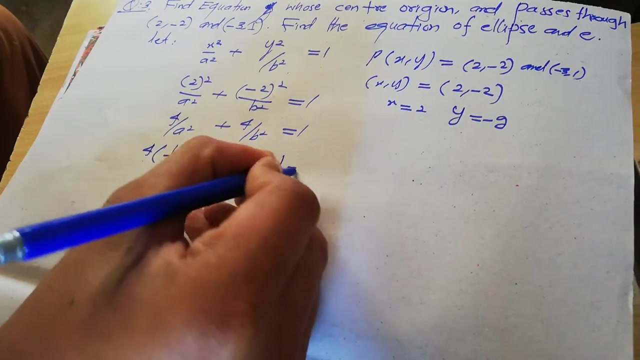 a square, y minus 2, whole square over b square is equal to 1. here it will be 4 over a square plus 4 over b square is equal to 1. now what we will do is separate it like this: 4 into 1 upon a square plus 4 into 1 upon b square is equal to 1. now take this as equation number. 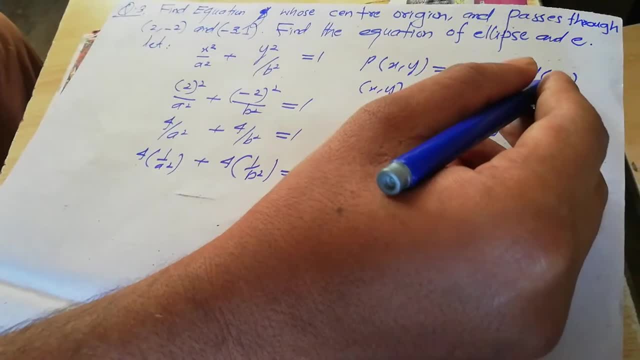 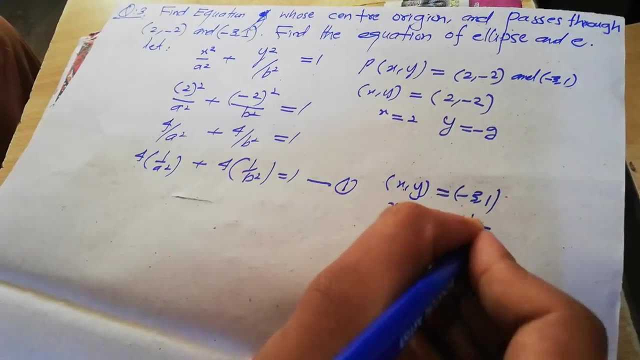 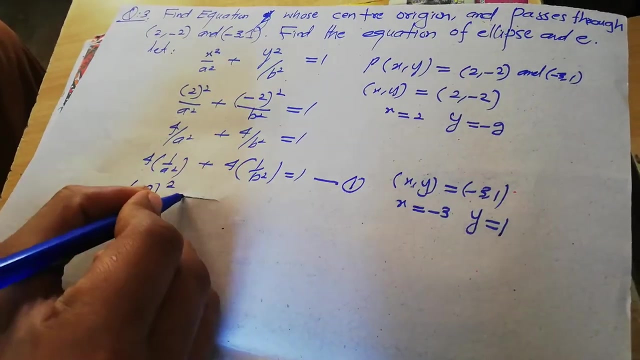 1. now the second point was minus 3 comma 1 means x. comma y will be equal to minus 3 comma 1. x's value is minus 3 and y's value is 1. now put these two values in general equation of the ellipse, which is x square, means minus 3, whole square over a square, plus y means 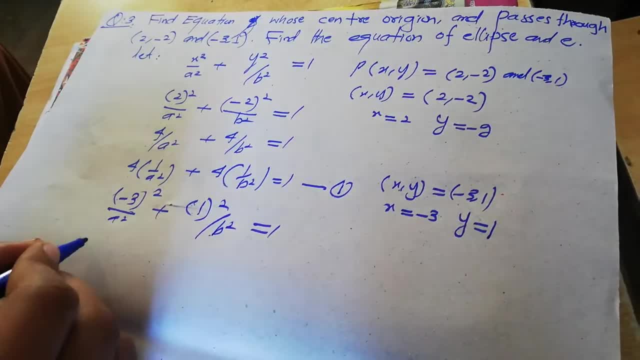 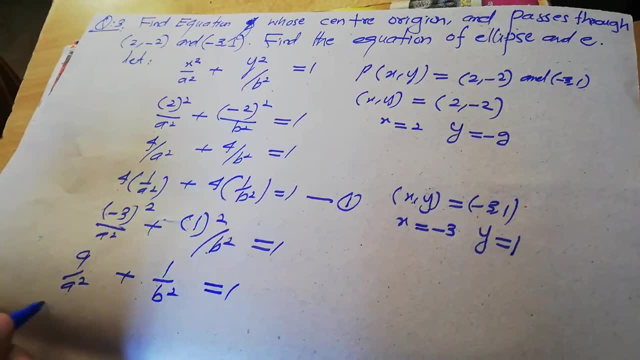 1 whole square over b square is equal to 1. here it will be 9 over a square plus 1 over b square is equal to 1. separate it like this: 9 into 1 upon a square plus 1 into 1 upon. 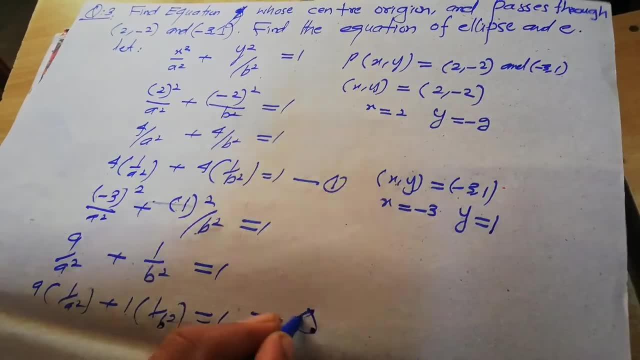 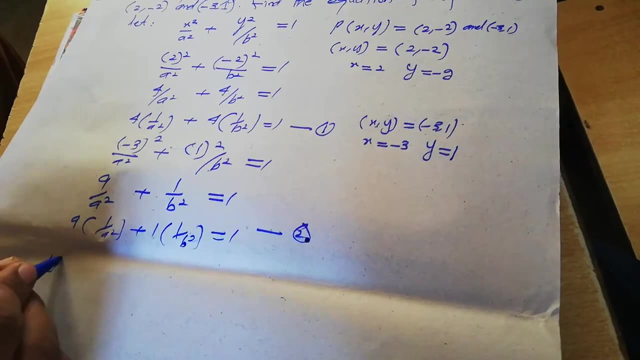 b square is equal to 1. so we will do this, equation number 2. now. equation 1 is done and equation 2. now. from here little bit of change will come. how that let x is equal to 1 upon a square and y is equal to 1 upon b. 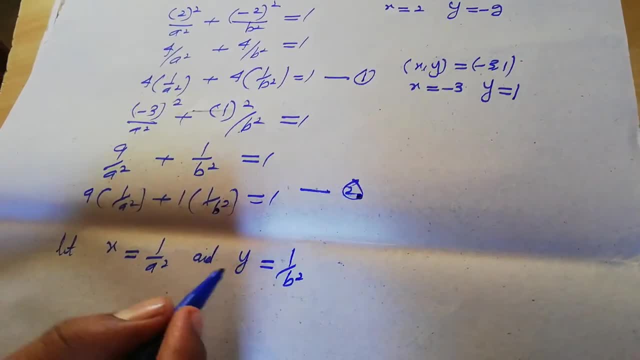 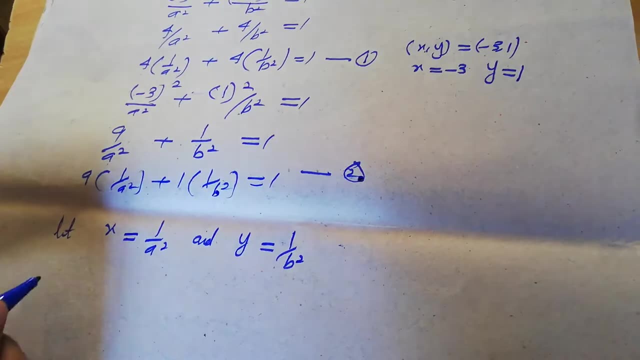 square when these two values, x and y, or we will put these two values here- that x is equal to 1 upon a square and y is equal to 1 upon b square. so equation 1 will be 4x plus 4y is equal to 1. 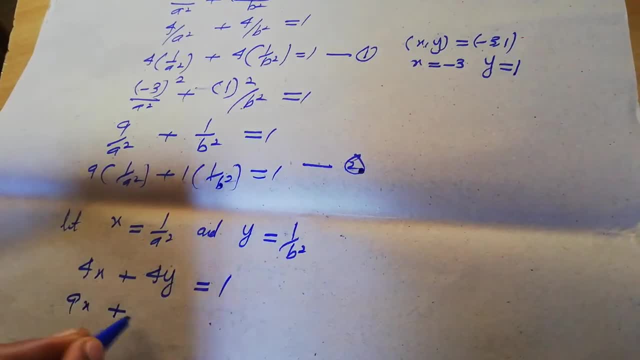 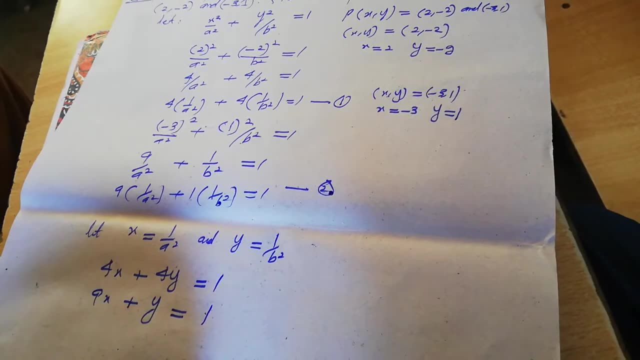 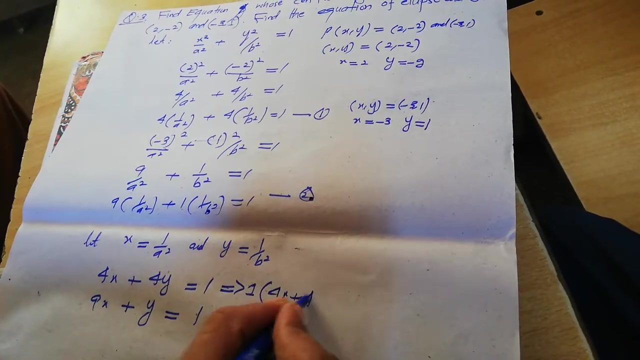 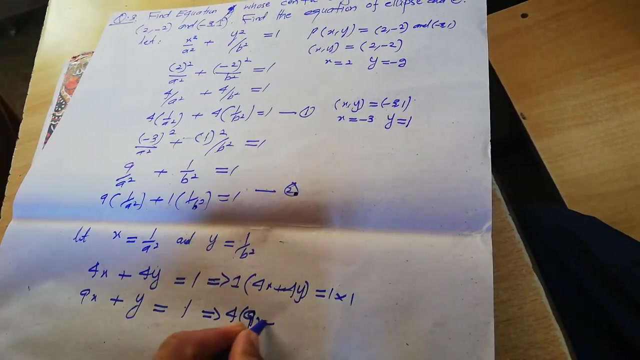 and equation 2 will be: 9x plus y is equal to 1. now, by comparing these two equations, how we will get the value of x and y. if we multiply 1 with equation, 2 means 4x plus 4y is equal to 1 into 1. and if we multiply 4 with equation, it will be 9x plus y is equal. 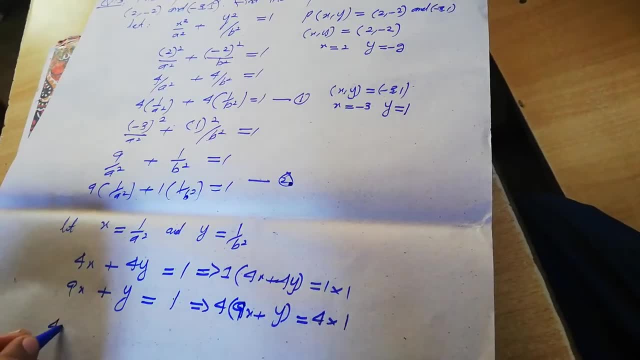 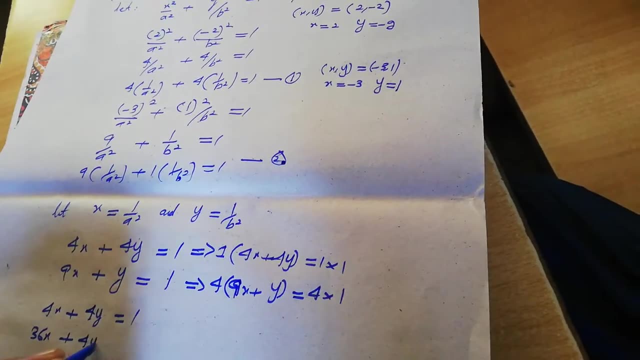 to 4 into 1, by simplifying it will be: 4x plus 4y is equal to 1 into 1. by simplifying it, 4x plus 4y is equal to 1, 4 times 9 is 36x plus 4y is equal to 4.. 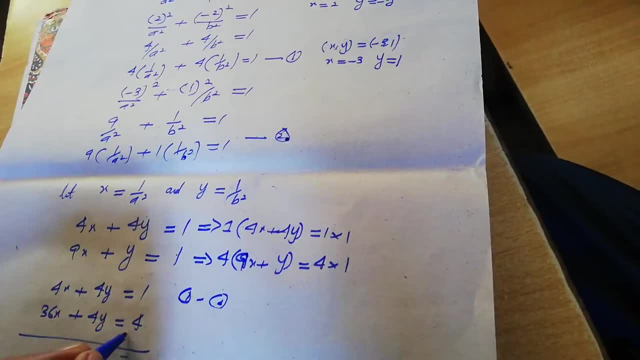 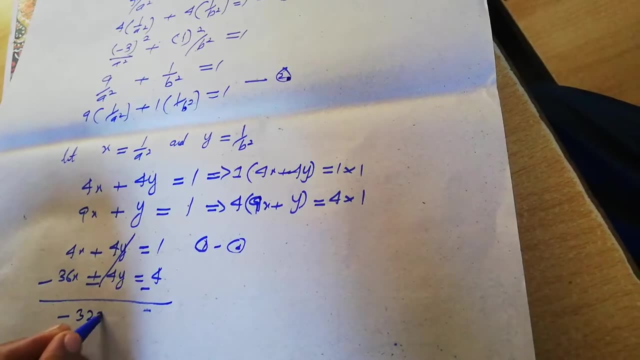 Now subtracting 1 and 2,, 1 minus 2, negative 4, negative negative. these two will be cancelled. Negative 36, positive 4,. what will happen? Negative 32x and negative 4, positive 1, negative 3,. 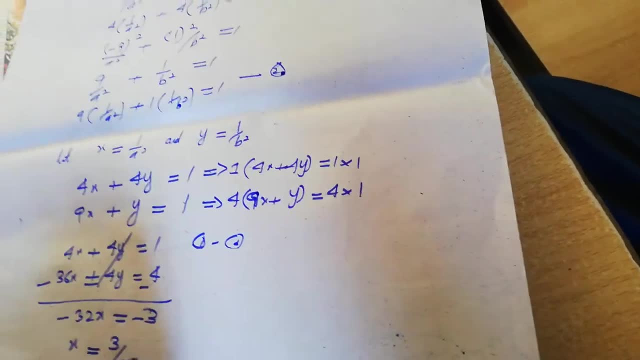 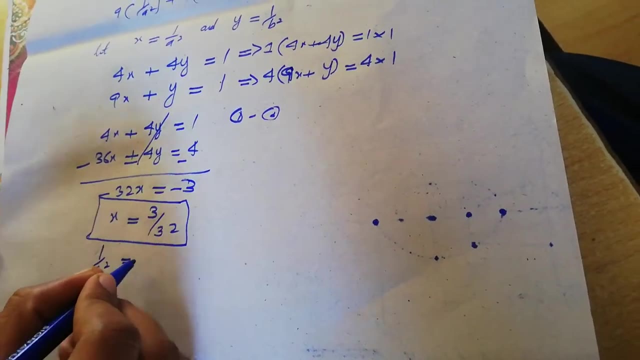 means the value of x is 3 upon 32.. Now this is the value of x. The value of x is equal to 1 upon a square. So 1 upon a square will be equal to 3 upon 32.. 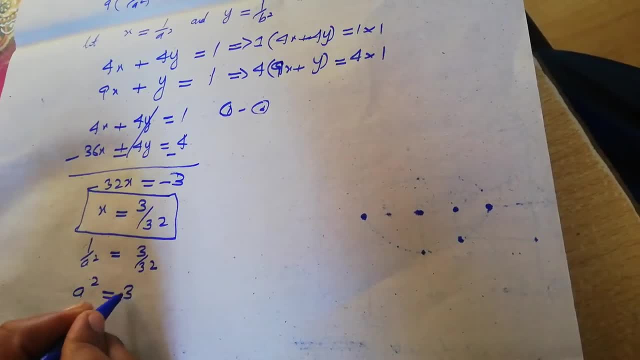 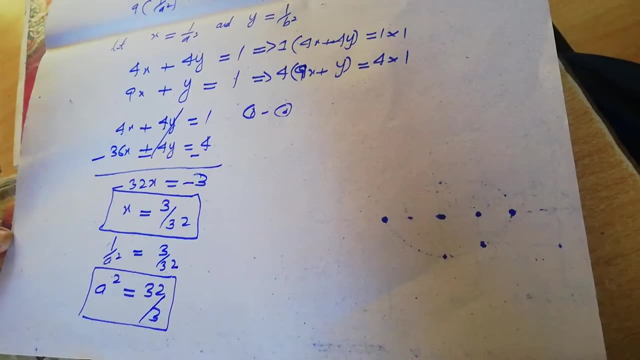 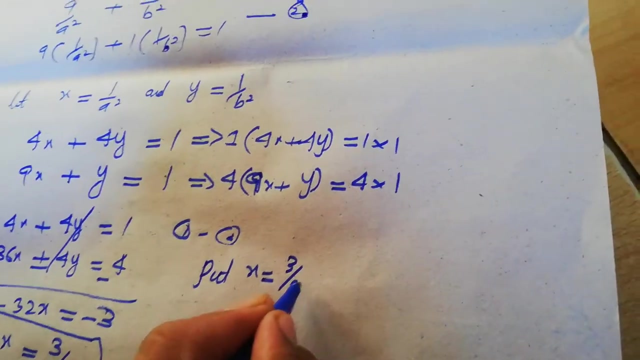 From here, subtract the value of a, What will be equal to a square 32 upon 3,. this is the value of a square. Now we will subtract the value of y, which is actually 1 upon b. square Put x is equal to 3 upon 32, and equation number 2.. 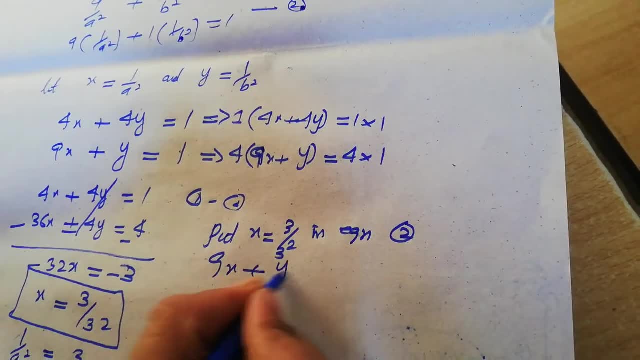 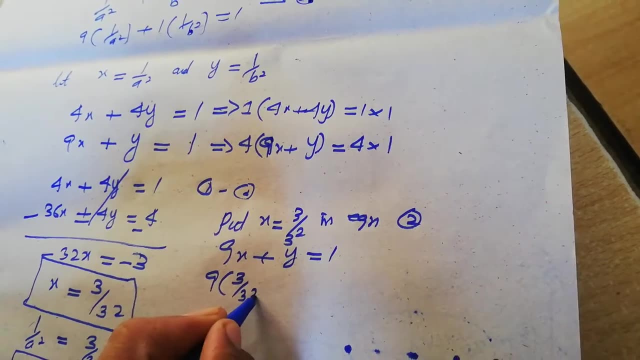 Equation number 2.. What is the value of x? 9x plus y is equal to 1.. What is the value of 9x? The value of x is equal to 30 upon 32 plus y is equal to 1.. 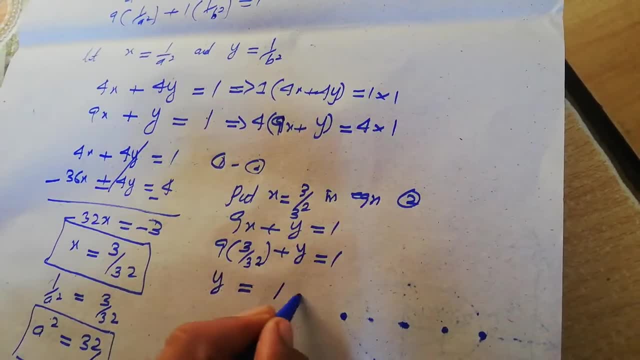 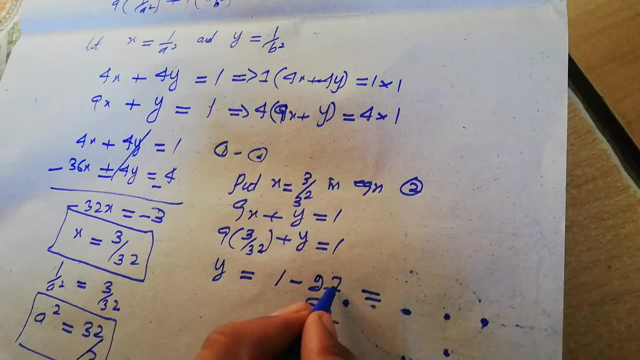 Now how will the value of y be? y is equal to 1 minus 27 over 32,, which will be equal to 32 minus 27, 5 over 32.. What is the value of y? 5 over 32.. 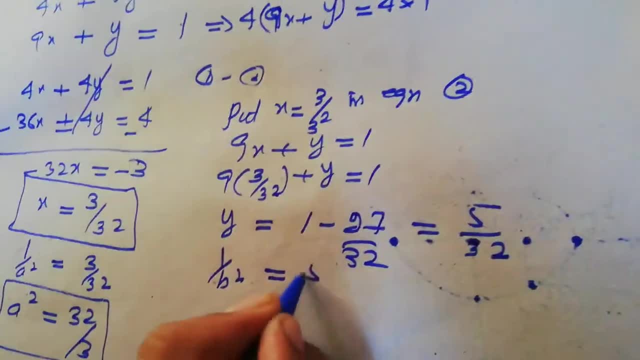 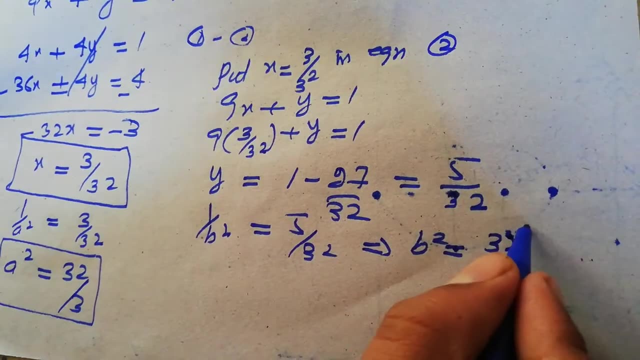 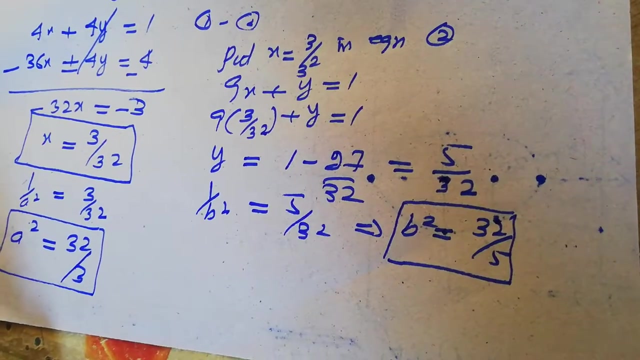 The value of y is equal to 1 upon b square plus 5 over 32 means b square is equal to 32 upon 5.. Now which equation will we put the value of a square and b square in In the general equation. then our equation of ellipse will come. 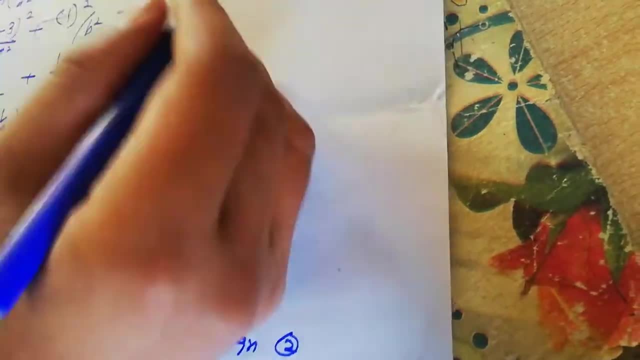 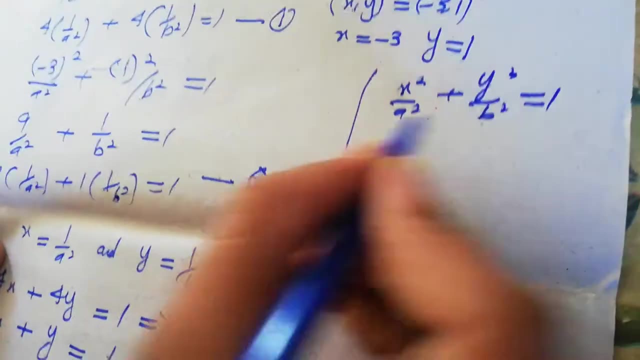 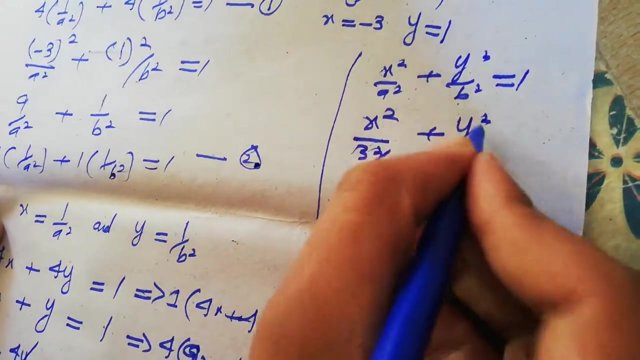 Which is the general equation. What is the general equation? x square over a square plus y square over b square is equal to 1.. x square over a square is equal to 32 upon 3, plus y square over b square is equal to. 32 upon 5 is equal to 1..